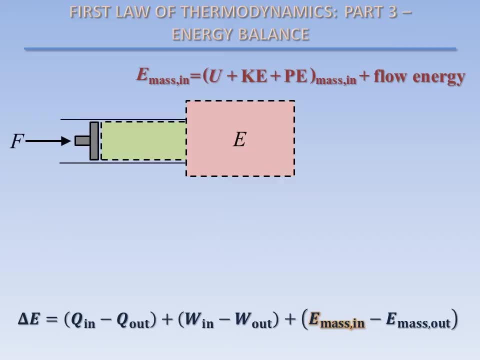 the energy required by an imaginary piston to push the mass into our system. Suppose the mass that will enter our system is at some pressure P and that it has some volume V. The force applied on the mass is equal to the pressure of the mass times its cross-sectional area A. 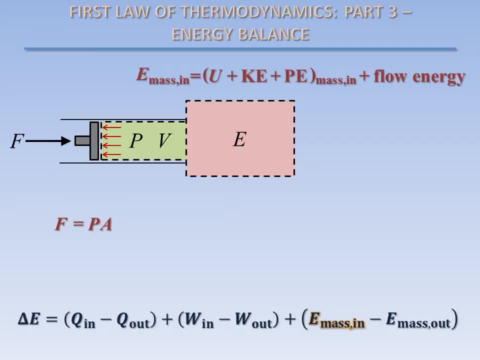 In order to push all of the mass into our system, this force must act over the entire length of the mass. L. The flow energy, then, is the force times the length. This can be expressed as the pressure times the volume. This flow energy is added to the total energy of the mass that will. 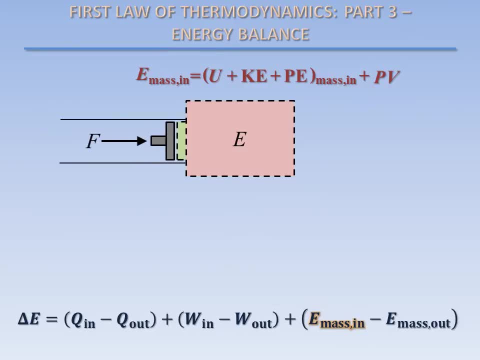 enter our system. We can rearrange this expression as follows: The internal energy of this mass and the flow energy required to push it into the system can be combined to form a new property denoted by the letter H. This property is called enthalpy. We can write the total: 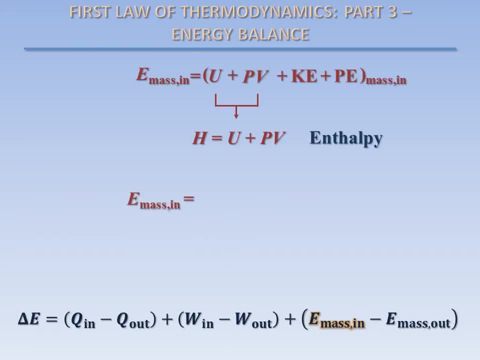 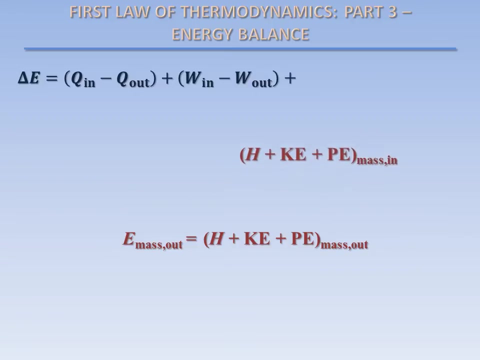 energy contained in the mass that has entered our system, in terms of enthalpy, as follows. A similar analysis can be performed on the mass flowing out of the system. We can now update our original energy balance with these new expressions for the energy flowing into. 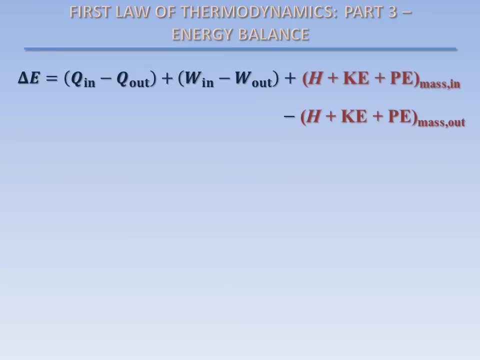 and out of our system with mass. We will rewrite the energy balance in a more general form as follows: The change in total energy of a system during a process which equals the change in the sum of the internal energy, kinetic energy and potential. 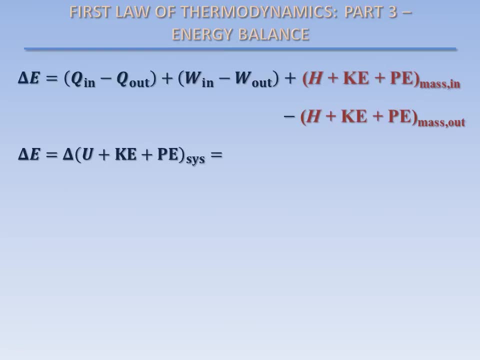 energy of the system is equal to the sum of all heat transfer interactions with the system, plus the sum of all work interactions with the system, plus the sum of all of the energy contained in the mass flowing into the system, minus the sum of all. 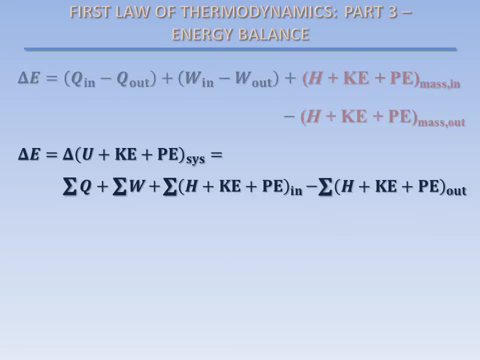 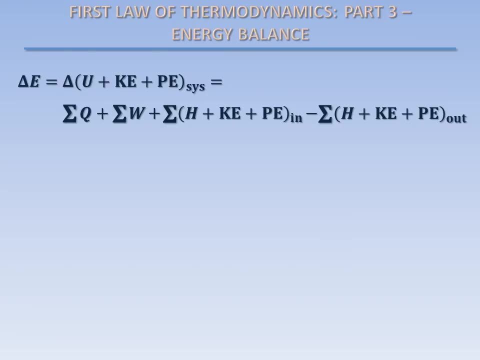 of the energy contained in the mass flowing out of the system. Let's make one more change to our equation. Right now, the total enthalpy of the mass entering and leaving the system are denoted by a capital H. This is an extensive property, which means that its value depends on the size or 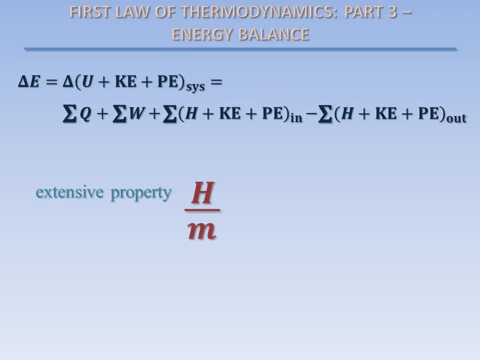 extent of the system. If we divide this by the total mass, we end up with a specific property. A specific property is an extensive property per unit mass. Specific properties are usually denoted by lowercase letters. Here the specific enthalpy is denoted by a lowercase h. 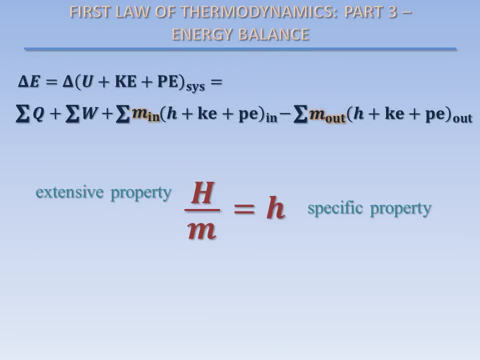 We can write our energy balance in the following form: where the total mass in and out is multiplied by the specific enthalpy, the specific kinetic energy and the specific potential energy of the mass flowing in and out of our system, This equation represents the energy. 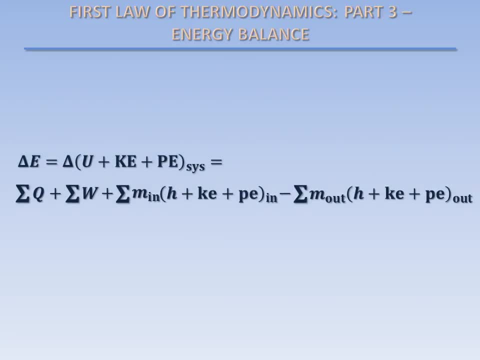 balance of our system. for some process, It is a mathematical expression of the first law of thermodynamics, or conservation of energy. 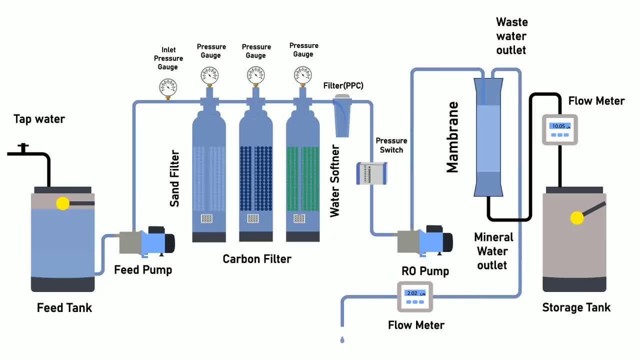 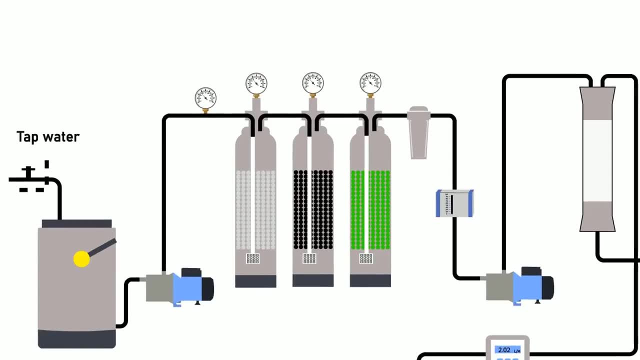 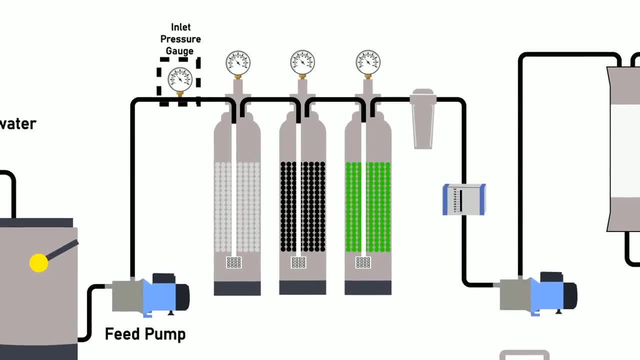 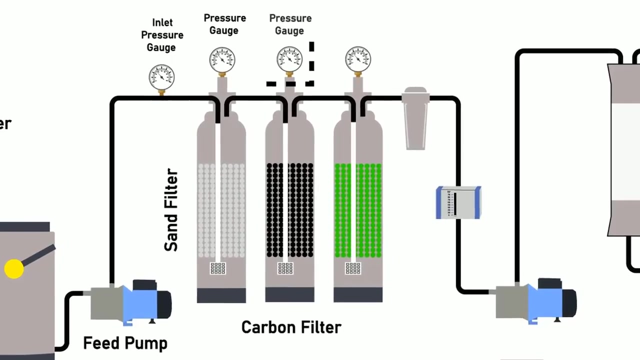 In this video you will learn the whole process of reverse osmosis RO plant. So let's begin with the parts of RO plant: Tap water feed tank, feed pump, inlet, pressure gauge, sand filter with the pressure gauge, carbon filter with the pressure gauge and water softener with the pressure gauge. 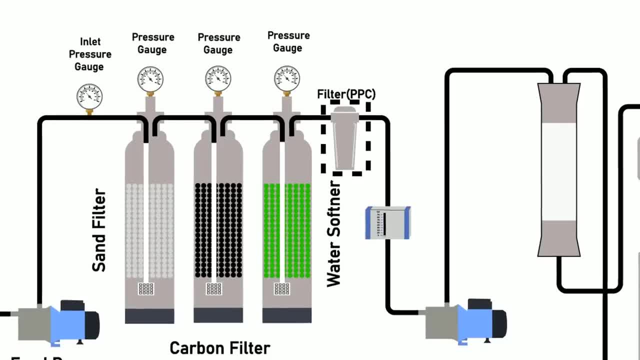 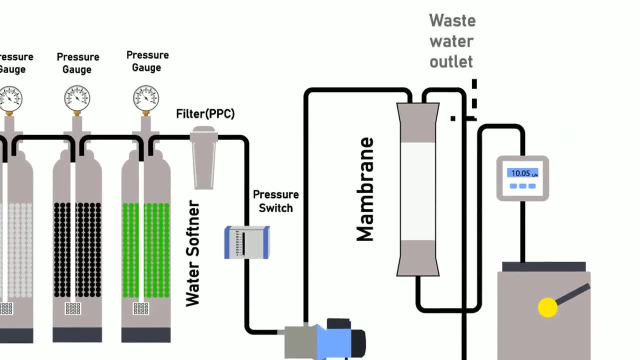 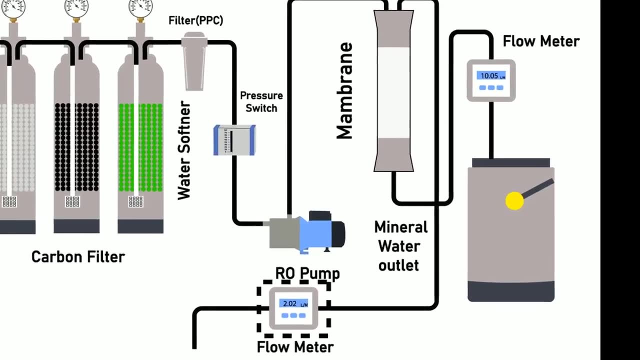 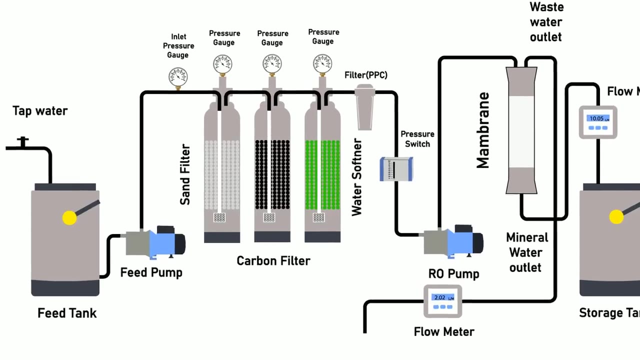 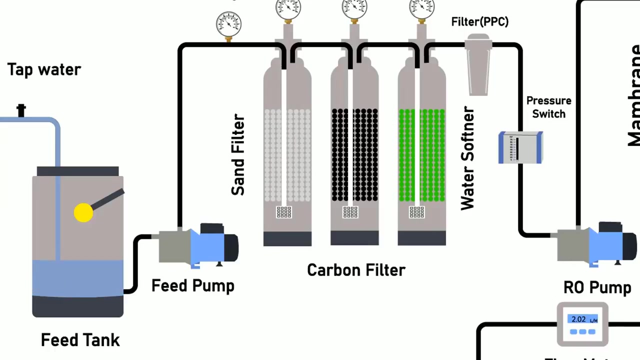 Then we have PPC filter, pressure switch, RO pump, membrane filters, waste water outlet, mineral water outlet, flow meters and storage tank. Let's begin the process. First of all, the feed tank is filled with tap water. The water filter sopr. 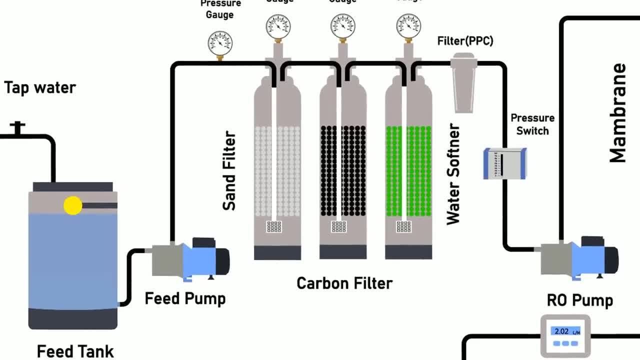 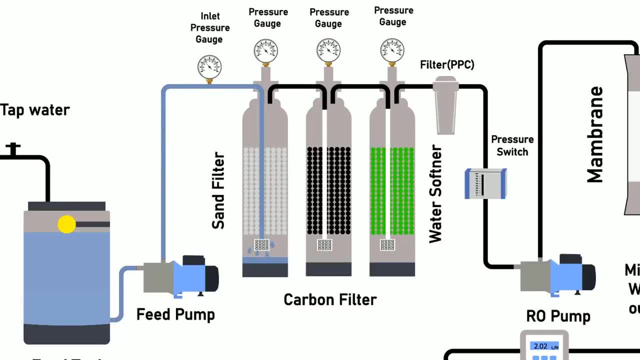 Further, the feed pump will transfer the water from the feed tank to the sand filter, Where all the particles separate from the tap water. The process occurs in such a way that water goes in and the opening is in the bottom of the tank. The water travels in.